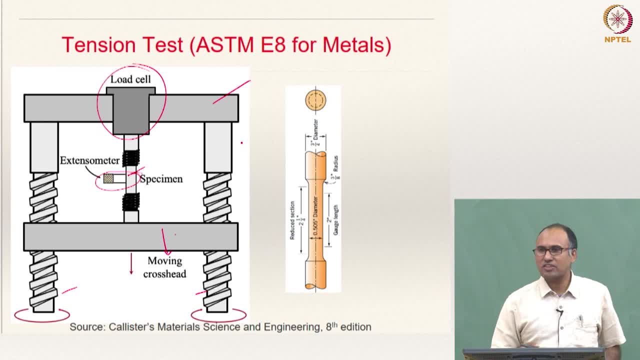 then it is not going to be precise because there is going to be some losses in the frictional interaction between the crosshead, as well as the screws and also the stiffness of the machine And hence, in order to measure- and also you have a gripping here and there may- 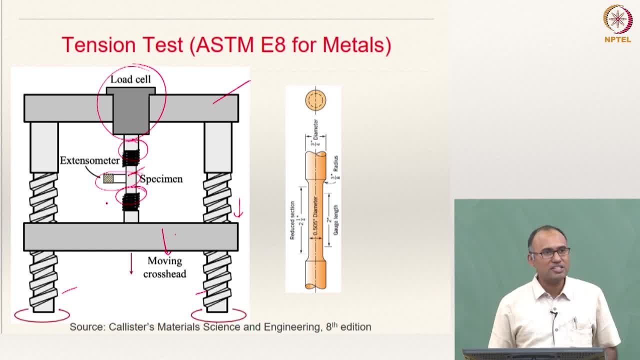 be some slip in the grips and so on. So to avoid this, you have to measure the stiffness of the specimen. To avoid all these errors in your measurement. you actually have a strain gauge, which is an extensometer, which is connected between two points, typically in the gauge section. 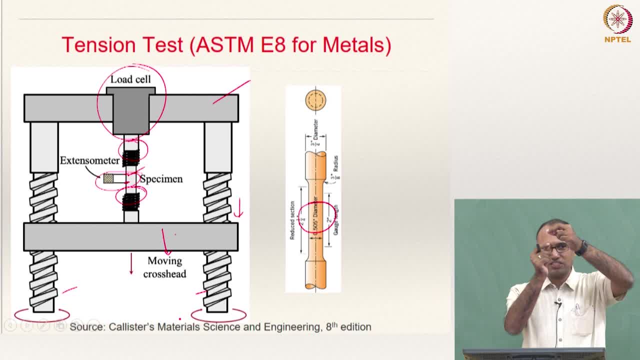 of the specimen so that you can actually measure what is the extent right. And this is a typical tension specimen and it is cylindrical in shape. but you also have tension specimens which are flat shaped- Okay, Thank you, And these are called dog bone kind of specimens, wherein you have the central region, which 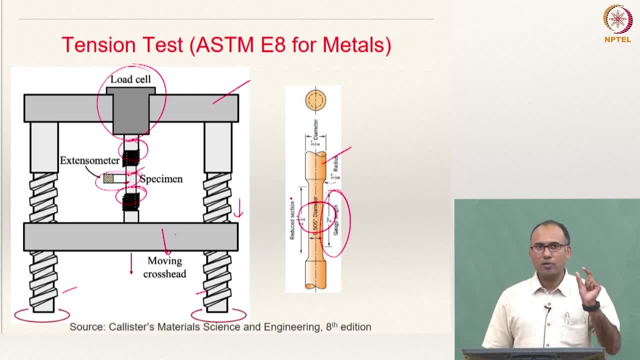 is called gauge section, having low, reduced cross section compared to the area where we grip the specimen using the crosshead right. So you will have gripper. depending upon the experiment that you want to do, you may have to change the gripper. 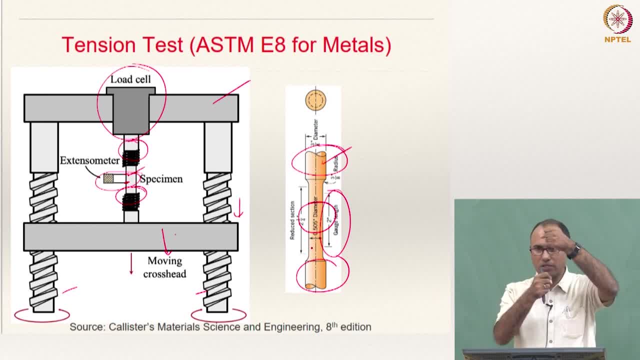 And depending on the geometry of the specimen. if it is a cylindrical specimen, then the grippers have to be of different kind as compared to when you have a flat specimen. Okay, So you need to buy these additional grippers as and when you want to change the geometry. 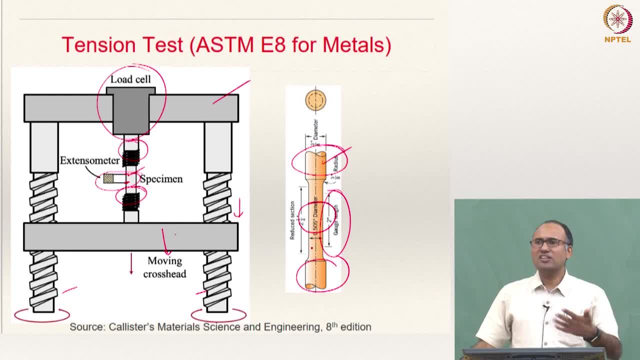 of the specimen that you want to test And similarly the same. it is called universal tension test or universal testing machine because you can do other tests as well, not only a tension test, but you can also do a compression test. If you have a fixture, appropriate fixture, you can do a shear test and you also can do 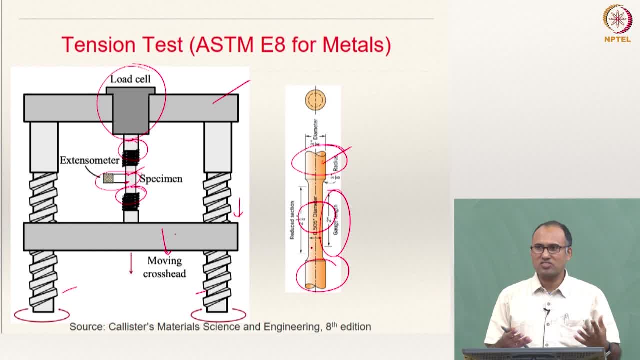 three-point bending. All that you need to do is the machine is the same. all that you will change is the fixture that is necessary for a particular kind of experiment, and that is why it is called UPM. Okay. And the most the critical thing is that when we have, whenever we are doing a test for 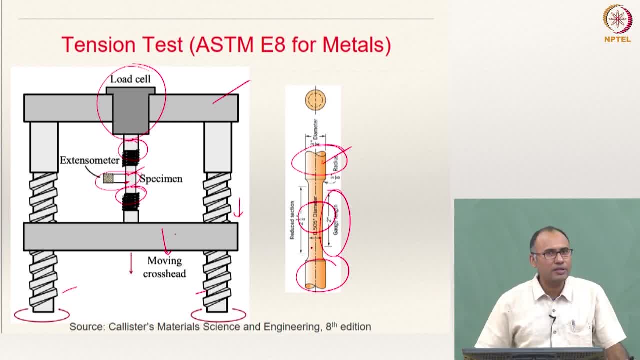 instance, a tensile test to measure the mechanical properties of the material. you need to ensure that the specimen is prepared according to certain standards. So this: for example, if you have a tensile test, you need to measure the mechanical properties. 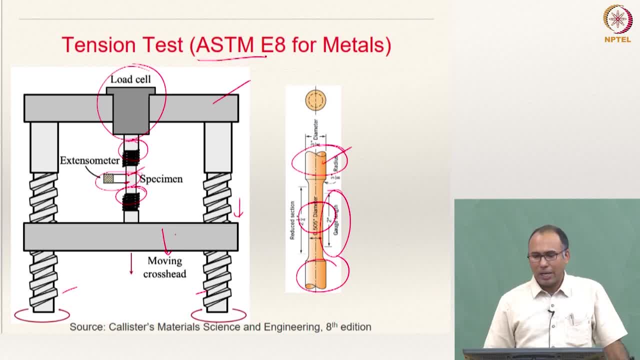 of the material. So this particular society called American Society for Testing of Materials, ASTM, has come up with several standards for each and every kind of a test. For instance, if you want to do a tension test on metals, okay. so ASTM-EH is the standard. 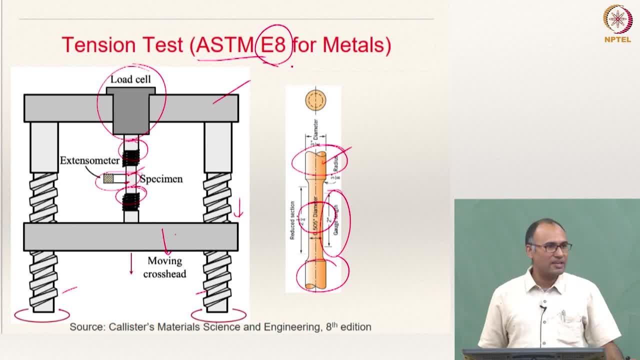 that one needs to use. So you need to go to ASTM standards and see the specimen specifications and prepare your specimen according to those specifications. The thickness, length, the ratios, if at all it is a cylindrical specimen, what should be the diameter of my gauge section, and so on, should be prepared according to ASTM standard. 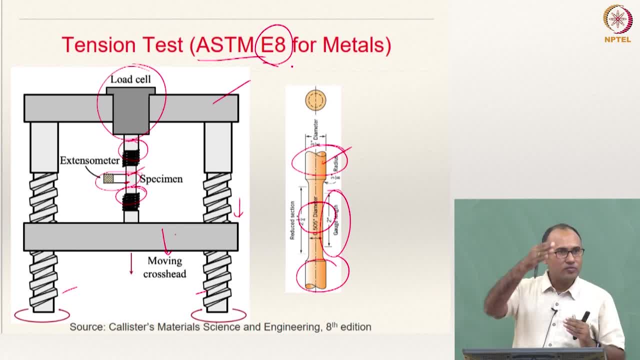 so that you can actually corroborate your results with the results available in the literature. Okay, So everybody who does this test will use the ASTM standard always, And sometimes it may be if you are working with a new kind of a material- it is possible. 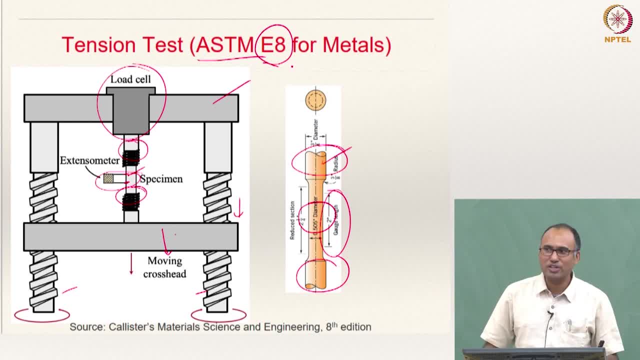 or probably not possible for you to make specimens according to ASTM standard, Then if you are doing so, when you are reporting your results, you need to mention what is your specimen size if it is not according to ASTM standard, because the results are going to. 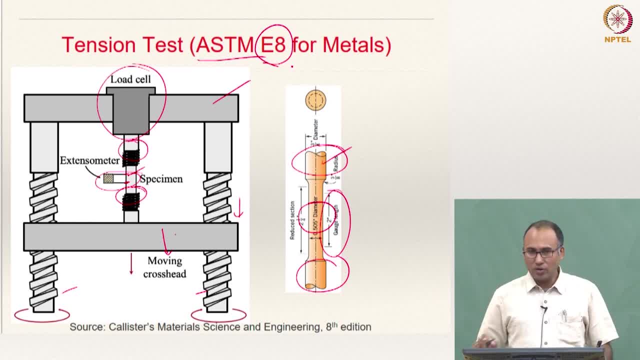 be different, And then somebody who is interpreting your results should be aware of the fact that there is a change in specimen geometry. Okay, Otherwise you will have conflicting opinions, Okay, So it is extremely important that the specimen geometry be specified clearly. 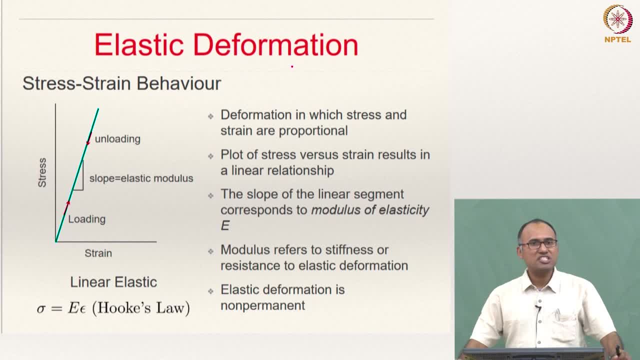 Okay, All right. So when you do this test, you probably have seen the load displacement curve and from there you can actually generate the stress strain curve. And I am here, I am showing individual parts of this stress strain curve and later we will. 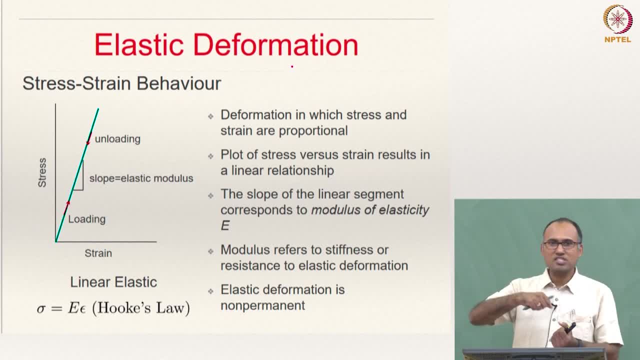 show the complete stress strain curve. So when you are loading the system initially you are, for instance, if you have done this experiment on metal Metal such as mild steel- you would have seen a linear elastic response. On the x axis you have strain and y axis you have stress. 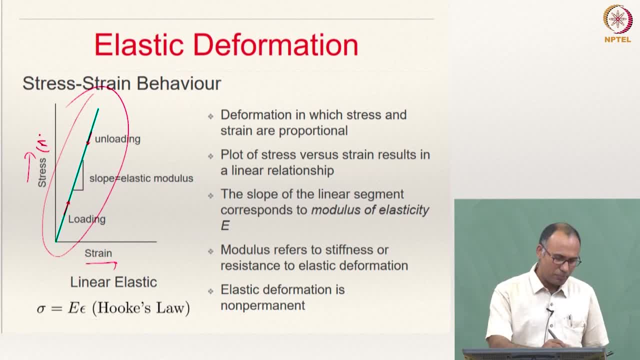 Okay, So stress, you have to say what are the units? Typically megapascals and strain units. What are the units of strain? It does not have unit because the definition of strain is change in length per unit original length. 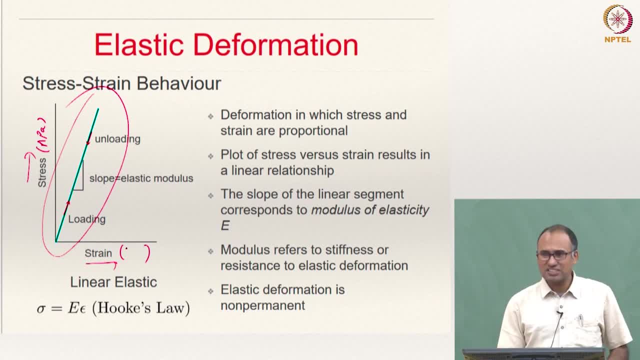 Right, Depending upon how you are defining your strain. So typically this is mentioned as strain, or sometimes you also can measure. mention this as a percentage of both are positive. Okay, So the initial response of the material is going to be elastic. 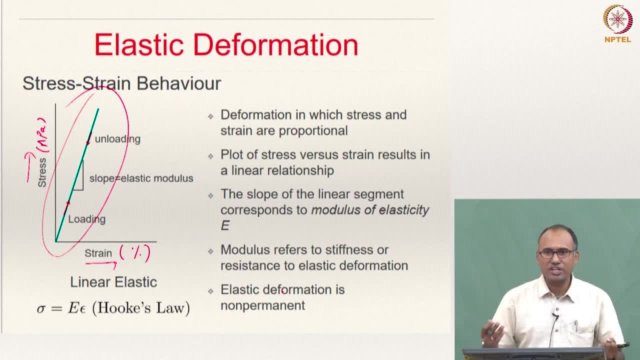 Before you actually going to deform material elastically, you have to elastically deform, Right, That is what you do. What is the meaning of elastic deformation? You are basically stretching the bonds between the material, Okay, Between the atoms, Right? 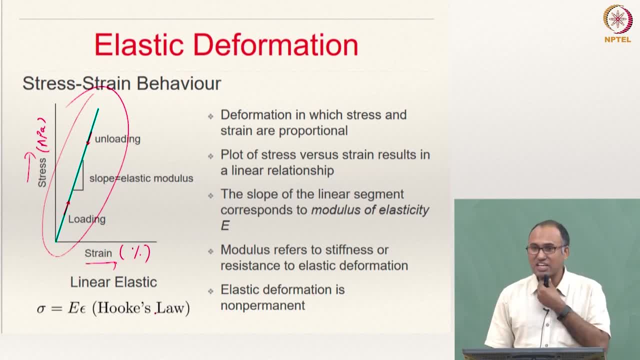 So in this region you have your stress and strain proportional to each other, Right? So here you have a linear elastic response, meaning the stress is proportional to strain. There is a linear relation between those two things And this is your loading direction and within the elastic regime, if you are unloading the 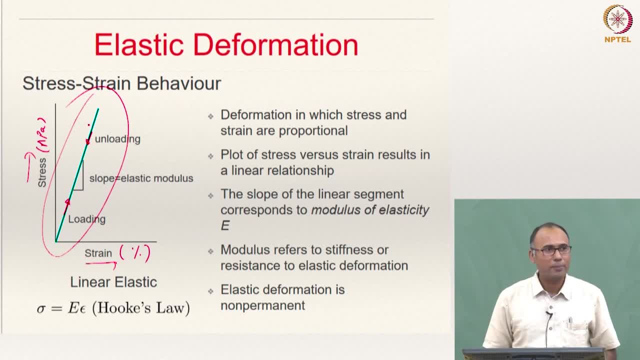 specimen. it goes back along the same path, Right. So the unloading direction is also the same And the slope of this stress-strain curve is what is called elastic modulus or Hengst modulus of elastic. So the E that we actually specify as the mechanical property is coming from the elastic. 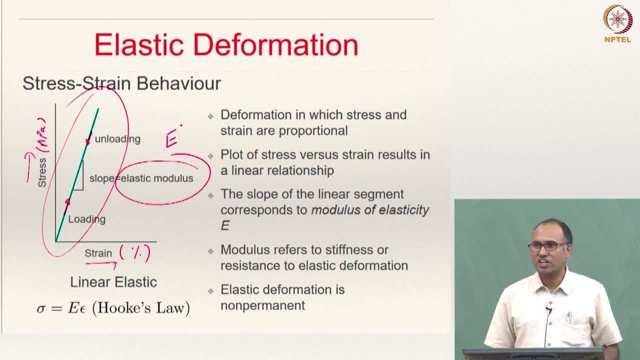 regime of your uniaxial tension. Okay, And, as we know, this elastic deformation is completely recoverable. It is non-permanent deformation, So as soon as you unload, you will go back to your original concentration, meaning zero stress state and zero strain. 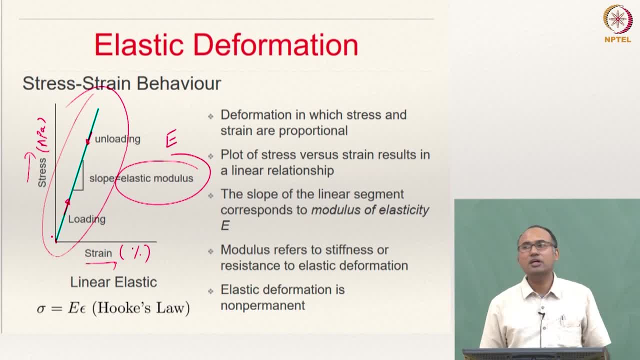 You will not see that the material is actually deformed, sometimes violated, Right. So the consecutive response that relates stress to strain in this regime is called Cook's law. is represented as sigma equal to E times epsilon, because it is a linear, elastic material. 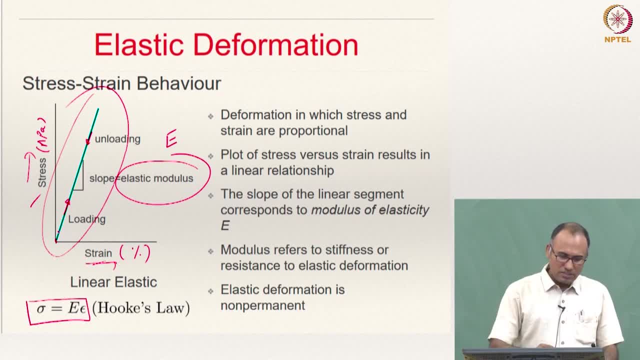 If it is non-linear elastic material, then this part will not be a linear fit, but it will be a non-linear curve and then your elastic modulus keeps on changing as you continue the loading Right. You will not have constant elastic modulus, but you will have varying elastic modulus. 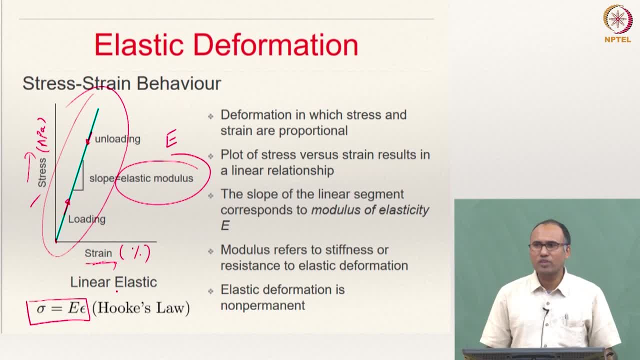 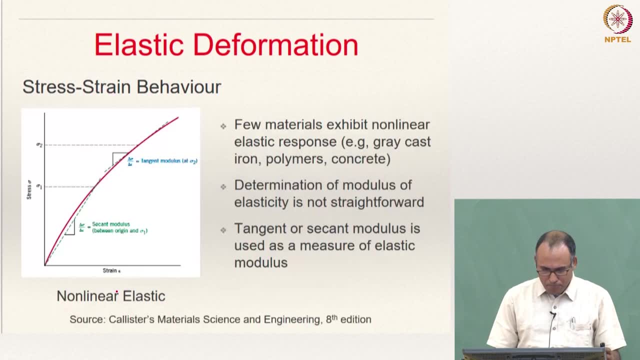 during the loading, And that is typically several times- we have flow such as behavior in elastomer polymer. Okay, So this is a typical non-linear elastic response wherein your slope of the stress strain curve keeps on evolving. So there are two ways to define the instantaneous elastic modulus. 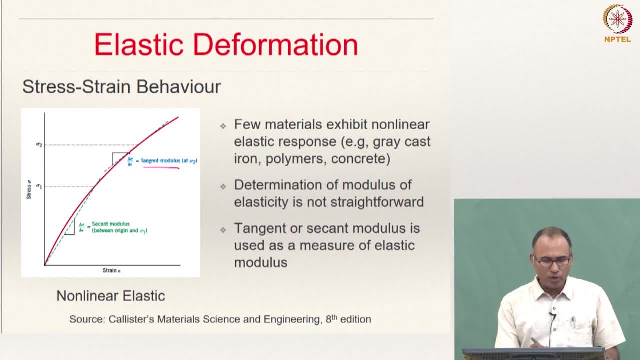 One is what you call tangent modulus. So if you are at a point given point, you draw the tangent to the line, to the curve at that point, And the slope of the tangent is called tangent modulus. And sometimes what you do is you can actually calculate secant modulus. 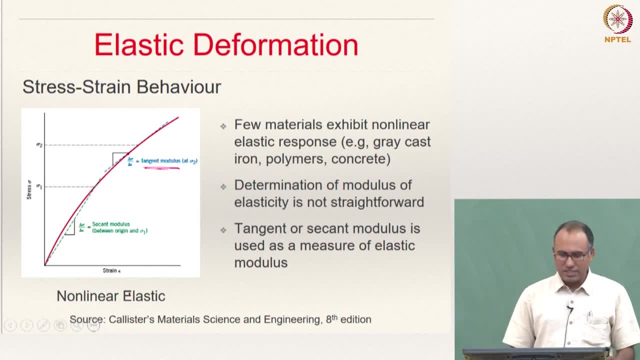 So you connect the line from origin to the point at which you actually want to find the slope, And then the slope of that line is your secant modulus, And this is usually preferred. but this is simpler, Right, Because you do not have to do any differentiation here. 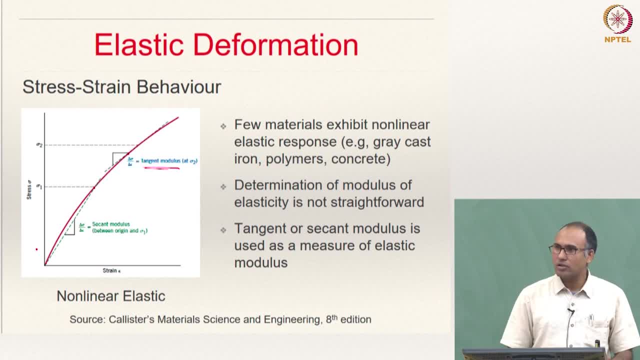 So computationally it is less expensive, but this is less expensive. Okay, So this is what you call the non-linear elastic modulus, Right? So computationally it is less expensive, but this is more expensive, but this is more. 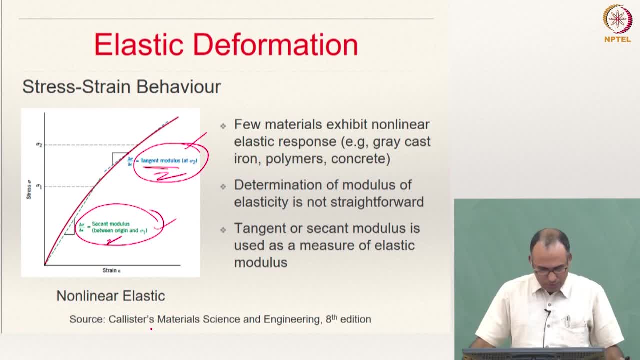 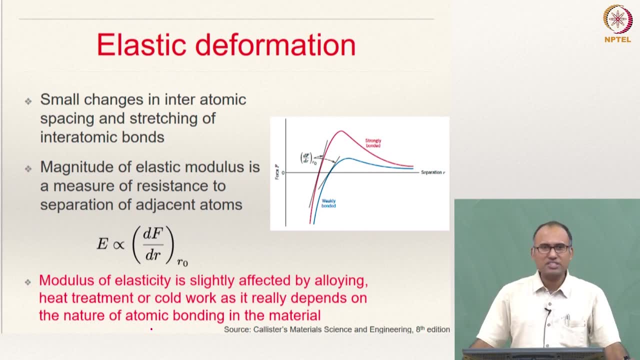 active, Tangent modulus is more active. Okay, And so what is this elastic deformation? Elastic deformation is actually nothing but the stretching of the bond, So the intradynamic spacing you are increasing as you are doing elastic deformation, but you are not breaking the bond. 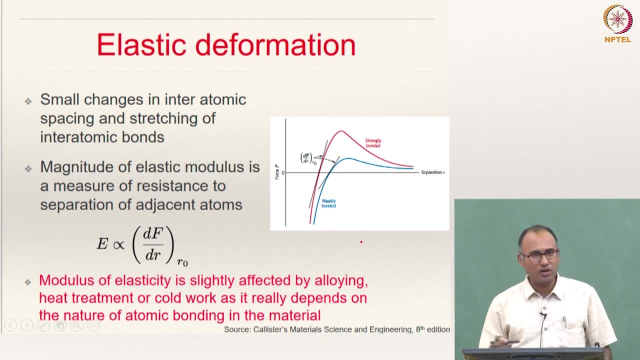 Okay, So this is the force separation response that you would have studied in your intradynamic bonding module, And from there you can actually say that your elastic modulus is a measure of resistance to separation of atoms. Okay, So, in other words, it is the stress of your stress-train curve which is the resistance. 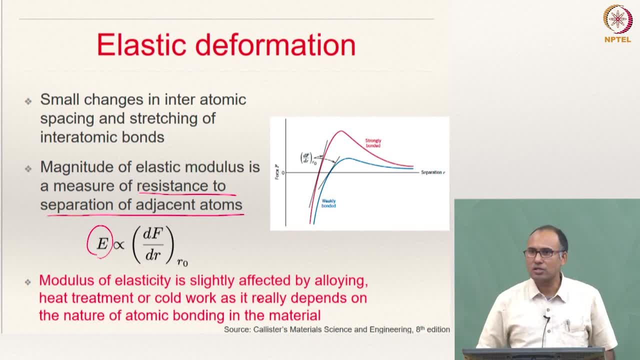 to separation of atoms. here I think you can see that when you are applying: Okay, So typically for materials, the modulus of elastic deformation is less than the stress curve. Okay, So the modulus of elasticity is very little affected, slightly affected by alloying heat. 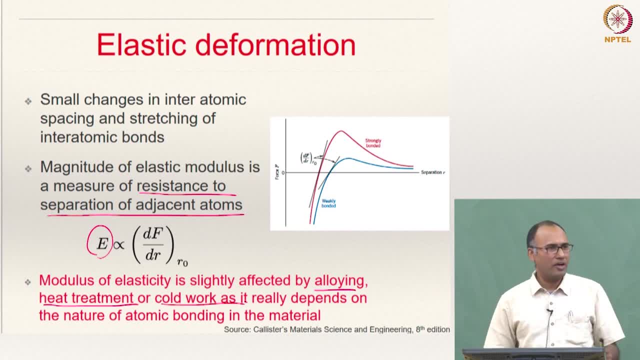 treatment, cold work. It is not significantly affected. little bit only changes and it really depends on the nature of atomic bonding in the material. As long as by doing these processes, if you are not changing the nature of atomic bonding, you are not going to change elastic bonding. 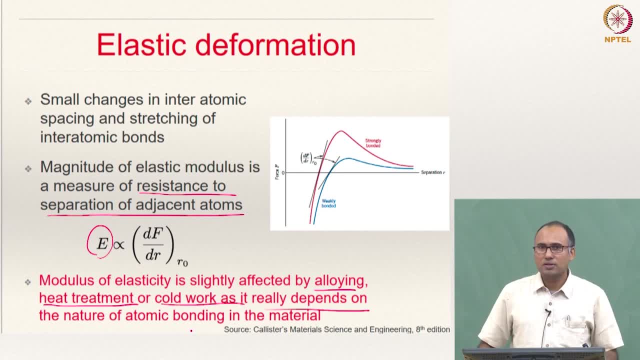 Okay, But as a function of temperature. what happens As a function of temperature? as you increase the temperature of the material, what happens to the elastic modulus? The elastic modulus changes, Right. So that is because we have seen this intradynamic separation force, separation law as a function. 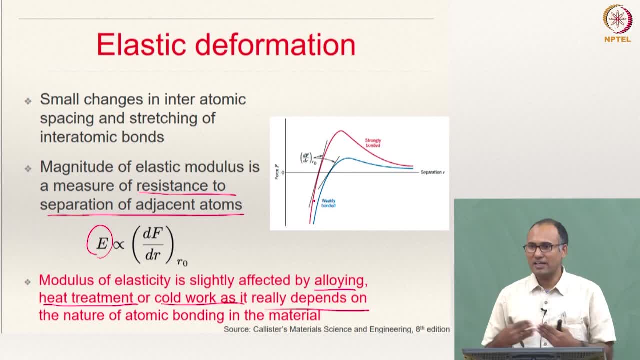 of temperature is going to change And, as a result, the slope of this curve is going to change as you increase the temperature, And hence you would see the temperature change. Okay, So you would see a difference in elastic modulus And many times, within certain range of temperatures, you do not see much of a change of elastic. 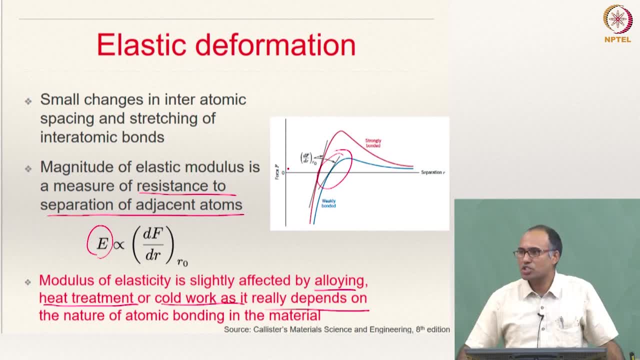 modulus, But beyond, at high, very high temperatures, you start seeing the effect of temperature on elastic modulus And hence, when you are analyzing the materials, you should, you should know what is the operating temperature And, depending on the operating temperature, you should decide whether you want to have. 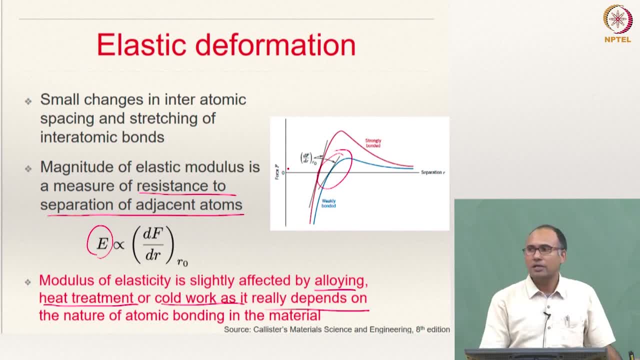 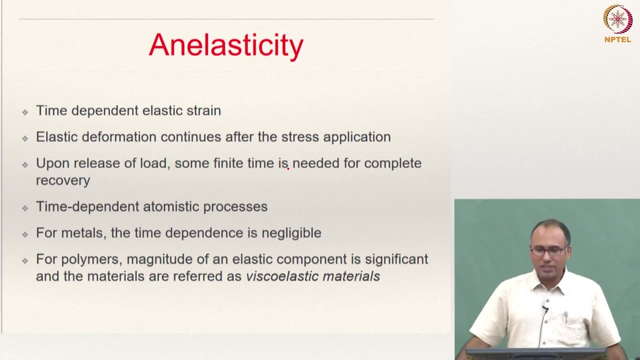 the effect of temperature included in the elastic deformation or not. Otherwise, you will be making a mistake in calculating the stress state of the material within elastic. Okay, And then you have another property called unelasticity, which is nothing but a time-dependent 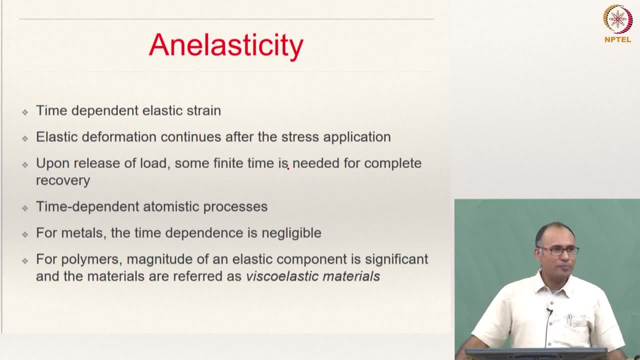 elastic. So what is the meaning of this? So, basically, when you are applying stress on a material, you apply a load. So you apply a load, So you apply a load. So what is the meaning of this? 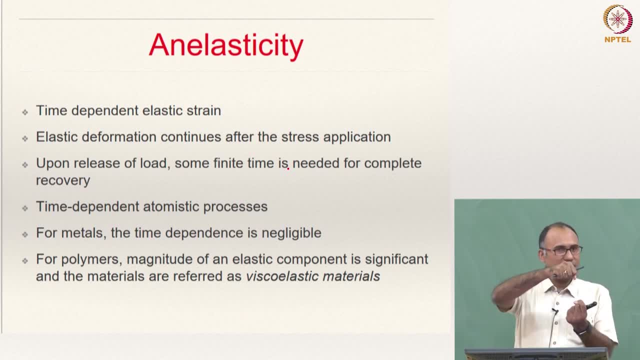 So basically, when you are applying stress on a material, you apply a load In the case of elastic deformation, and if you are holding that particular load, then strain remains constant unless you further increase the stress Right. But in the case of unelasticity, even after maintaining the stress constant, you may observe. 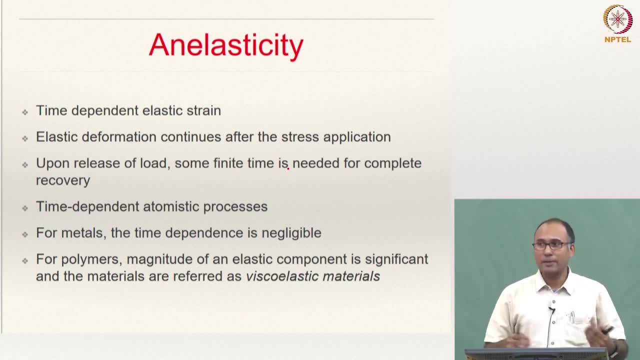 some strain, continuity, Okay, So, as a function of time, this material actually starts to deform, even though you are not increasing the magnitude of the stress that is applied And at the same time, in the case of elastic deformation, the moment you remove, you unload. 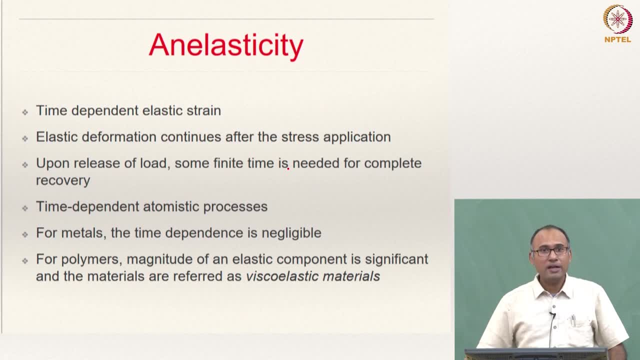 the specimen, it comes back to its original configuration immediately. There is no time factor involved, Whereas in these kinds of unelastic materials you unload the specimen to zero stress, but then the specimen takes some time to come back to its original configuration. 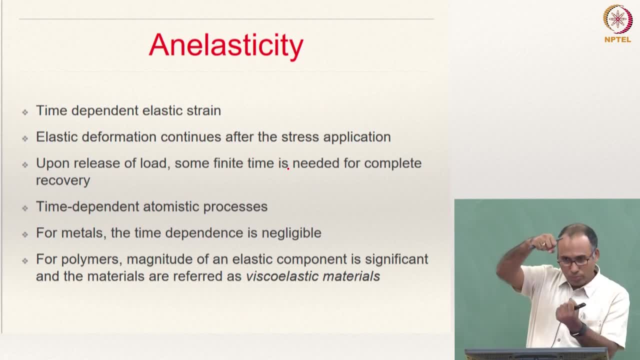 So in the case of unelasticity, you need to increase the stress, even though you are holding that particular load at the moment. Okay, So when you are applying stress on a material, you apply some stress Right And at the same time, you are holding that specific load at the moment. 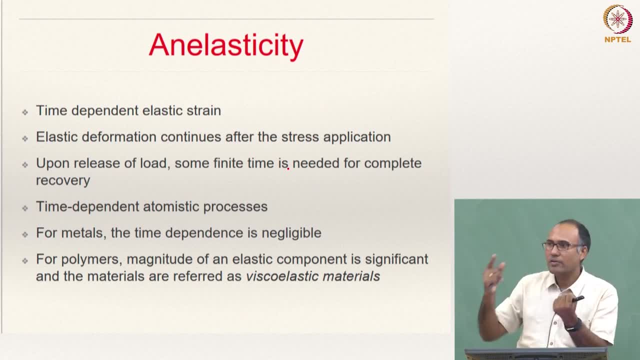 So, as a function of time, you apply a load, So you apply a load, So you apply a load. Okay, And you apply a load, Whereas in these kind of anelastic materials you unload the specimen to zero stress. 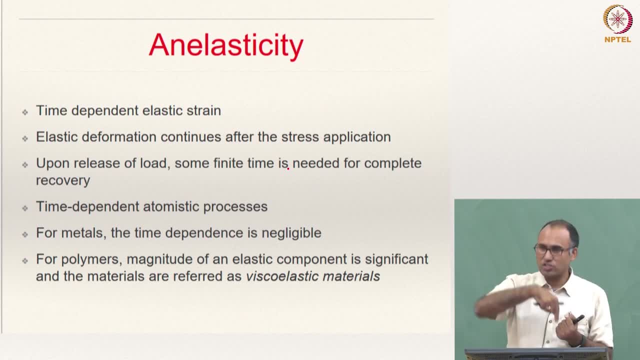 But then the specimen takes some time to come back to its original content. It will come back but it may not come back immediately. So that means there is a time factor involved. so after sometime it will come back, So immediately. if you would measure you might see that there is some crash to the specimen. 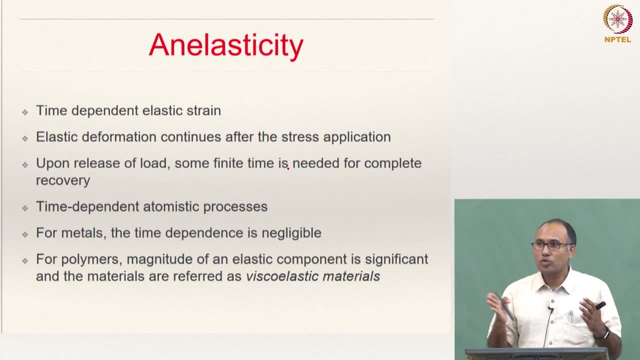 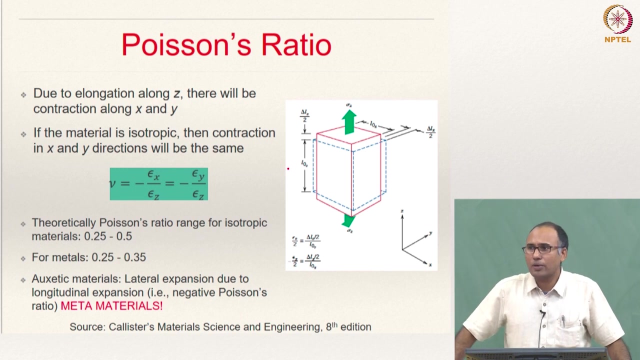 there is some permanent deformation But that permanent deformation slowly reduces as you wait for longer time. For metals usually it is negligible, but for polymer this is one of the important deformations. So that is about one of the important mechanical properties called elastic modulus of the material. 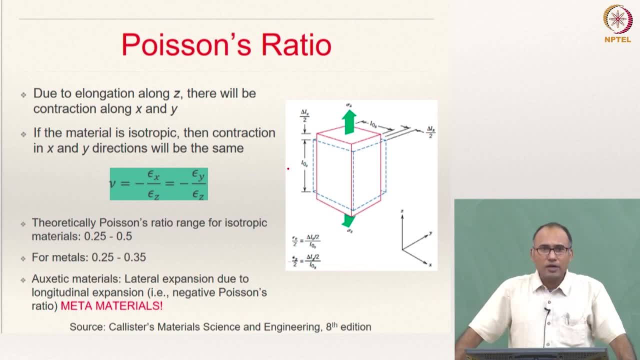 How do you go about measuring the elastic modulus For linear elastic material? it is like this: For non-linear elastic material it is going to be constant. For non-linear elastic material it will be a function of stress state or strain that you have imported in the material. 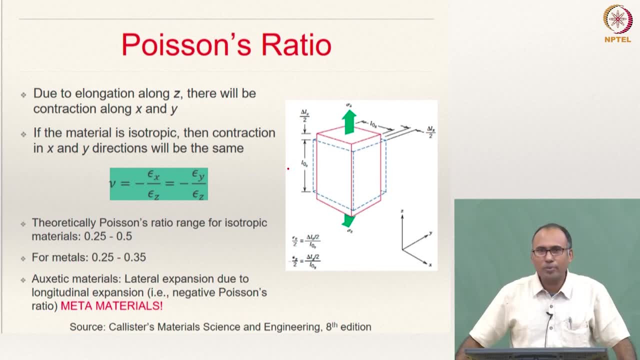 And the next important property of the material that we need to focus on is Poisson's ratio. So what is this Poisson's ratio? If you are deforming a material normally in one direction, then let us say it is getting elongated. 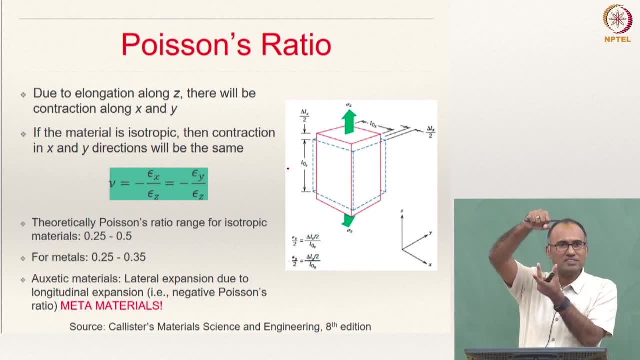 In the lateral direction it contracts. Why does it contract In one direction? you are elongating in the lateral direction. the material has to contract. That means in this direction. if the strain is positive in the lateral directions, the strain will be negative. 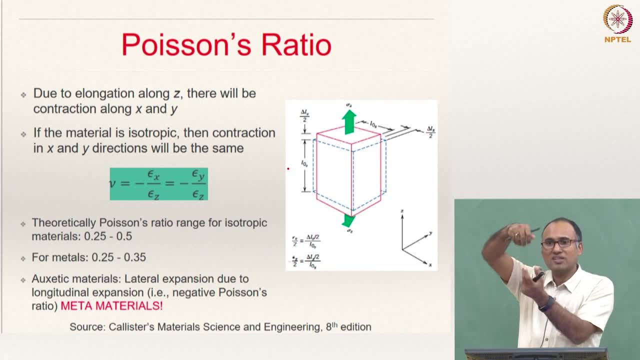 Why does it have to be negative? Because volume has to be constant. Right, Because volume has to be constant. you are not adding any additional volume. So the Poisson's ratio is defined as negative of lateral strain by longitudinal strain. So if you are taking the specimen and if you are loading the guy in the z direction- epsilon. 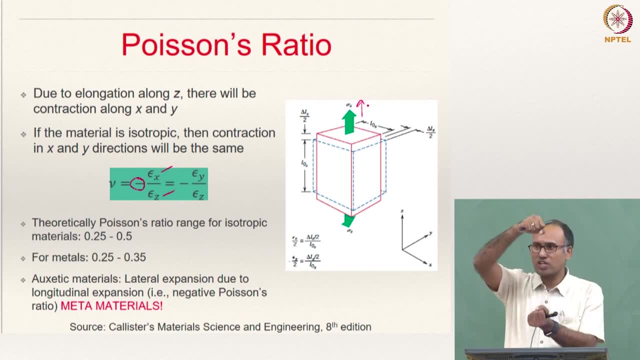 z is the longitudinal strain, and the lateral strain will be epsilon x or epsilon y. Right, So you can define your Poisson's ratio actually as nu xz and nu xy. That is minus epsilon x by epsilon z. That is minus epsilon y by epsilon z. 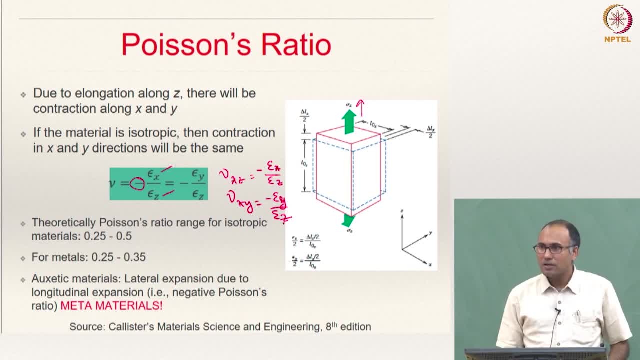 But typically for isotropic materials these two values are going to be same. Okay, So nu is defined. for an isotropic material, You can simply say lateral strain, You can simply say lateral strain by longitudinal strain. But if it is an anisotropic material, it is not going to be a single number. 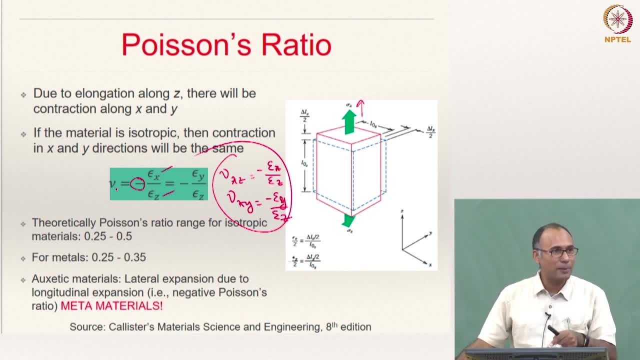 It depends on the direction in which you are actually measuring. Okay, So the most important thing to remember is that there is a negative strain sign here, And hence your Poisson's ratio will always be positive, Right? So, theoretically, the Poisson's ratio range for isotropic material is 0.25 to 0.5. 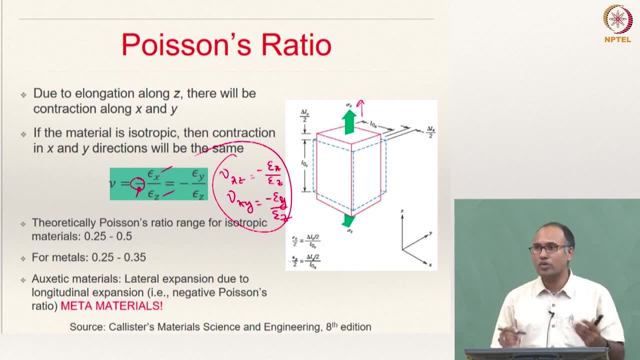 And for metals the Poisson's ratio is 0.25 to 0.5.. So the Poisson's ratio for isotropic material is 0.25 to 0.5.. So the Poisson's ratio for isotropic material is 0.25 to 0.5.. 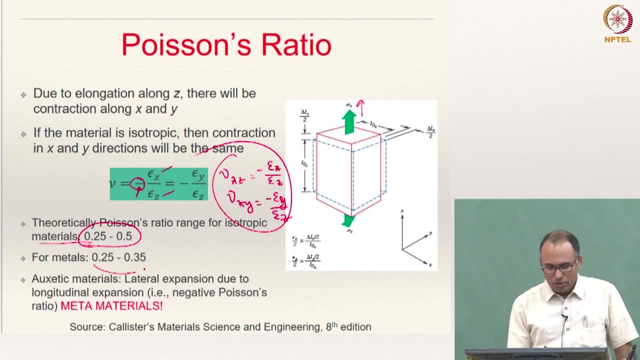 So the Poisson's ratio for isotropic material is 0.25 to 0.5.. And for metals 0.25 to 0.35.. But you can actually show that by using energy argument the Poisson's ratio can be a max. 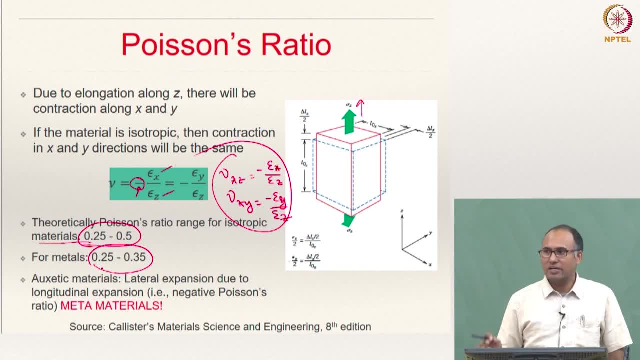 at most it can be plus 0.5, and it can actually go to negative 1.. So it can be actually between minus 1, less than or equal to epsilon, less than or equal to 1.. You see, So not a mistake. 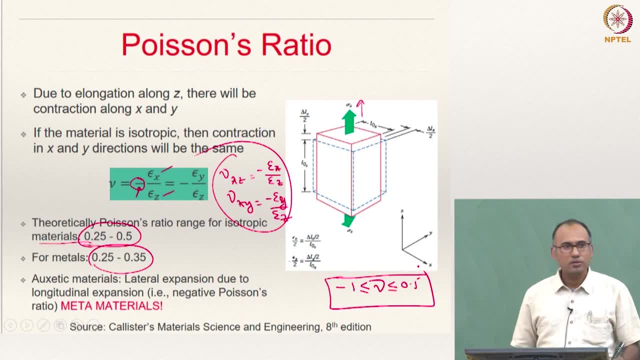 That is the range of Poisson's ratio. Poisson's ratio value you can obtain theoretically. But what is the meaning of we said we just now discussed, when you are pulling a guy in this direction, then what should happen in the lateral direction? 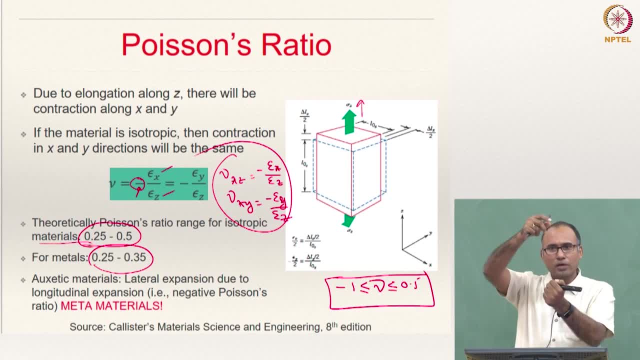 It should contract Right. As a result, you can only conceive a positive Poisson's ratio. So what do you mean by negative Poisson's ratio? What do you mean by negative Poisson's ratio When you are pulling the guy in this direction instead of contracting in the lateral direction? 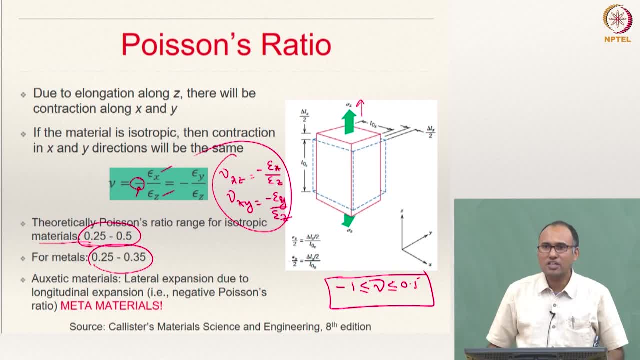 the material expands, then such a material will have negative Poisson's. So normally crystalline materials, you will not observe this negative Poisson's Always. you are somewhere. that is why this is the range that we need to go. But there are new class of materials called auxetic materials, which show lateral expansion. 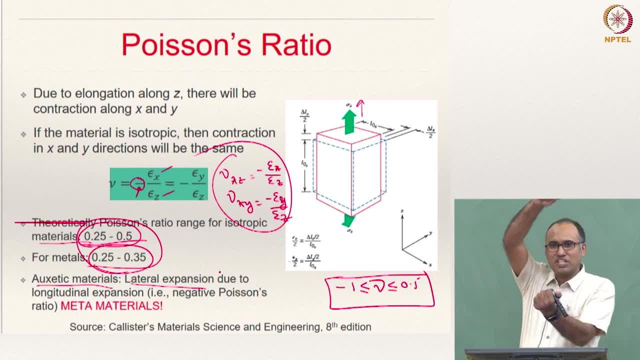 due to longitudinal expansion. So when you are applying tension in this direction, in these materials, you observe also expansion in the lateral direction. That means your Poisson's ratio is negative. Such materials are called metamaterials. they are general class of metamaterials. 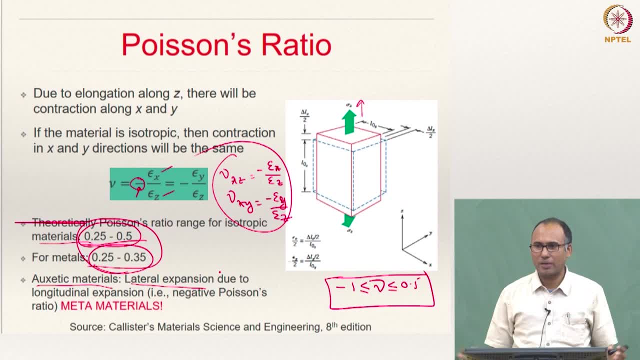 Auxetic materials are a subset of the big class of metamaterials, So this is the recent evolution in terms of material design. So what can they offer? They can offer tremendous new possibilities in terms of mechanical deformation because people have, for instance, several biomedical devices, which, for instance, the stents that 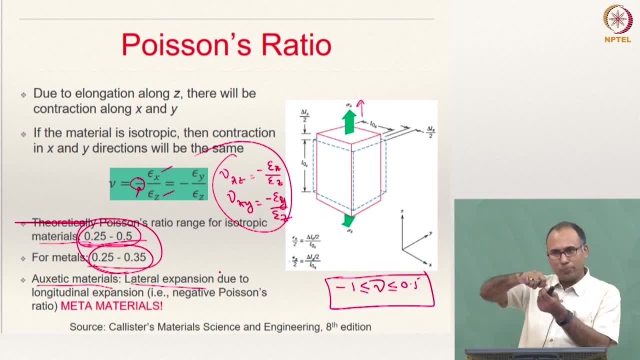 you send into arteries. You want to actually pull them. You want to pull them At the same. when you are pulling them, you want them to expand later so that they can fit in the artery. So that kind of structures can actually be now designed as a reality. 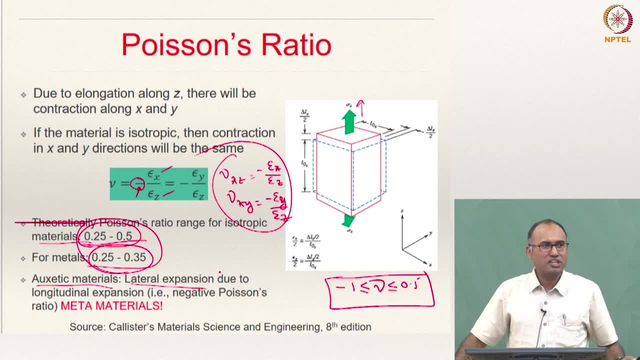 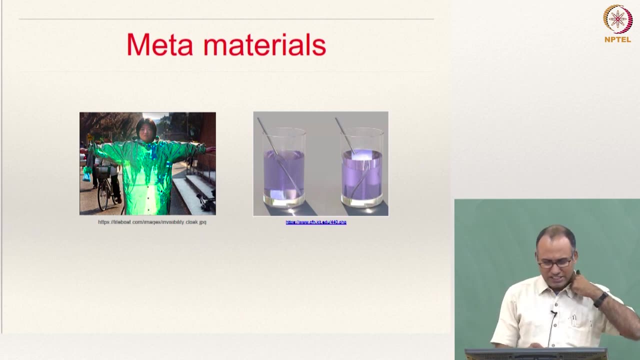 It was not possible, say, 20 years ago, but today we can very well nicely design these structures from mechanical engineering point of view. But you also have other interesting metamaterials. So you see this guy, this is what is called invisibility. 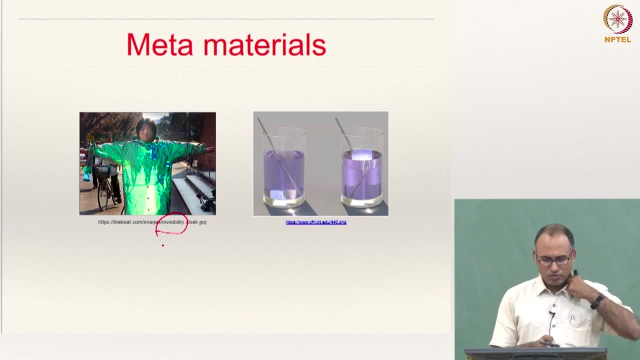 So you can see this guy wearing a shirt. You must have seen this in Harry Potter. So it is not a fine- vexing thing- People have actually demonstrated invisibility- but means that there is basically optical flow. So you play with your refractive. 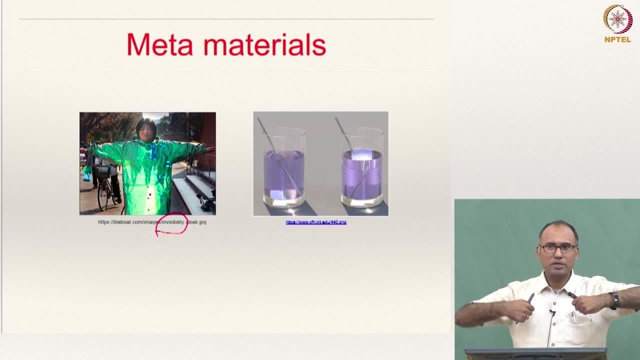 So the fact that you are able to see me standing here is because you lived in a very, very deep, vast place. Now, This is the way that I want you to imagine me. You have to be able to imagine. I will show you what that means. 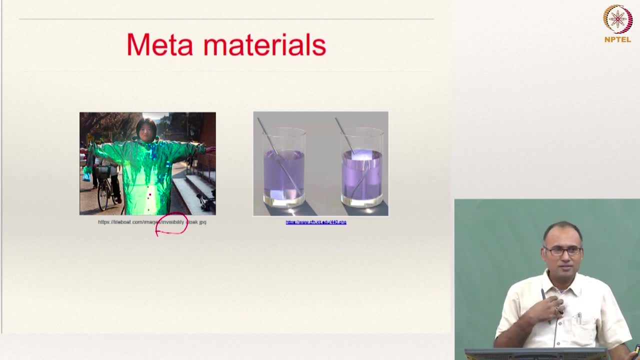 This is what it looks like. Here is how it looks, Because the light rays that are falling on me are reflected back and, as a result, you are able to see me. otherwise, you will not feel my action right. What if I can? what if I block the reflection of light wave from my direction? right, or? 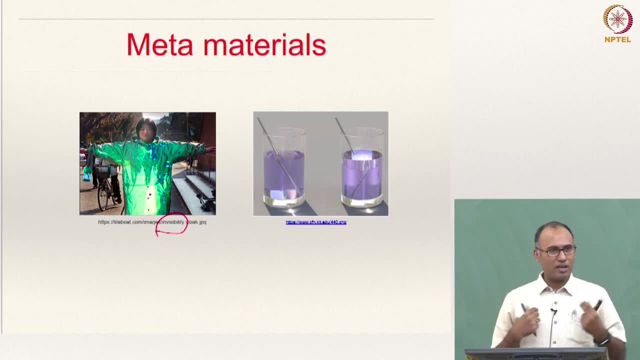 I will, rather than reflecting in that direction, I will send all the light that is falling on me in these ways, and then it is not actually going and hitting in your eyes right, and hence you think that I am not, although I am not, is not it? 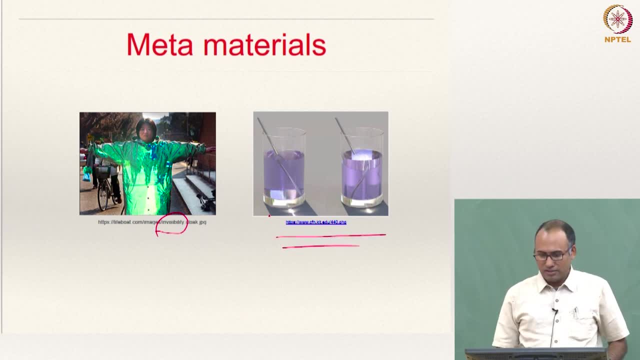 So, similarly, you see this guy, this is normal right, the left hand side is normal, the right hand side is not normal. So you are playing with your refractive index of the material and you make your negative refractive index and then you actually can show something which is naturally not broken. 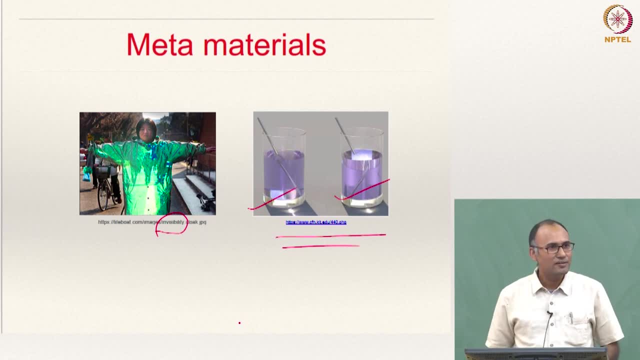 as if it is two different things, right? So this is. people have actually theorized this thing- optical cloaking and all quite some time ago- but now people are able to make design materials which can change refractive. Now people are talking about acoustic clock. what is the meaning of that? 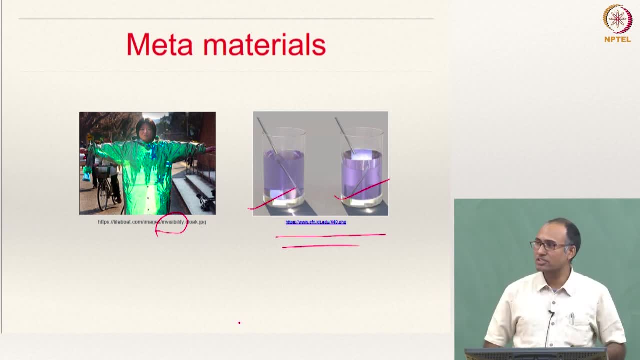 So suppose you want to have a window, so something I do not know. it is not yet a reality today. so I want that window, I want it to be a window. So I want that window, I want it to be open because I want the air to flow in, but I do not want to hear the 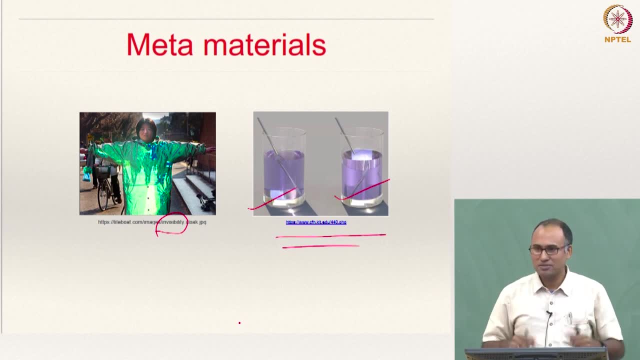 noise outside. is it possible? right? What I want is basically, I want to filter out certain frequencies, but that means the noise- that is, whatever noise that I am going to have- should not be coming through the window, but I only want air, right? 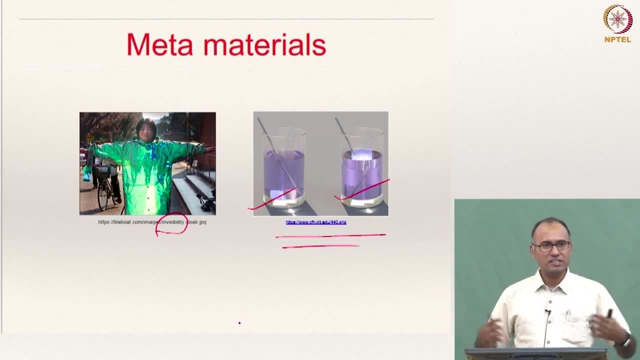 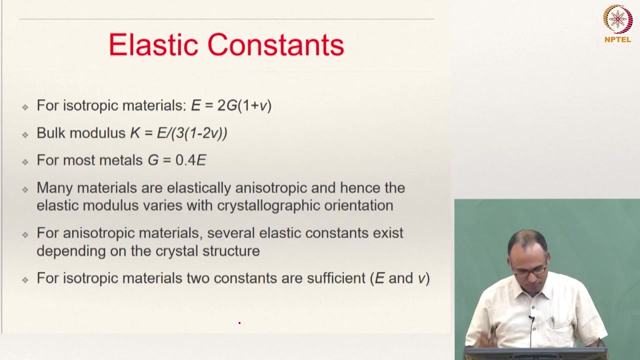 Similarly, there are infinite number of possibilities If you can think about new kinds of materials. all these things are today possible and one can actually make several things which are science fiction. in your Harry Potter movies or in several Indian mythology, We would have thought about them as science fiction, but today you can actually make them. 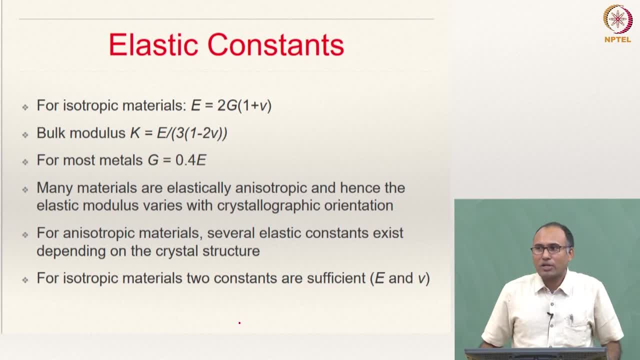 very well, All right. So we have discussed about elastic constants: E elastic modulus- mu- Poisson's ratio. We have discussed about E elastic modulus- mu- Poisson's ratio. We have discussed about E elastic modulus- mu- Poisson's ratio. 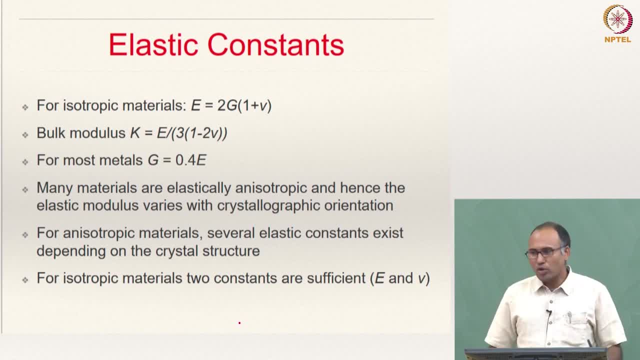 We have discussed about E, elastic modulus, mu, Poisson's ratio. Why This is only true for isotropic materials. You just need to describe their elastic response. You only need two constants for an isotropic material to describe the elastic response. But if it is an isotropic material, you will require more number of constants and hence 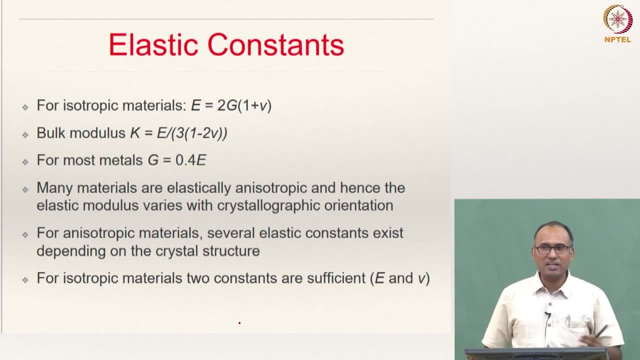 you need to do more experiments. So for isotropic material you can actually measure the Poisson's ratio and elastic modulus using. how many experiments Have you tried measuring Poisson's ratio of your mild steel specimen? you did not try. You can actually try. right, because you have measured the longitudinal strain and at the 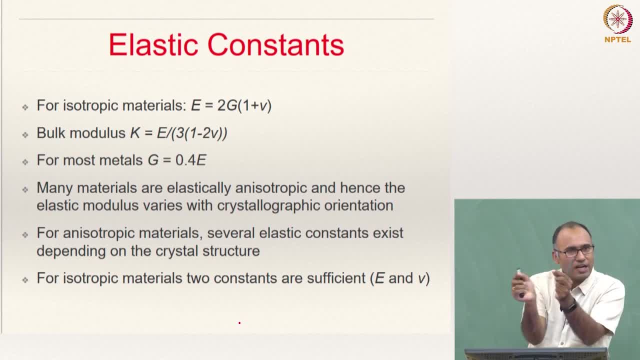 same time you can put a strain gauge in the opposite direction, and then you would have measured the lateral strain, is not it? So the elastic modulus and Poisson's ratio could have been measured at the same in one single. So you also have the relation between other elastic constant like shear modulus, G, bulk. 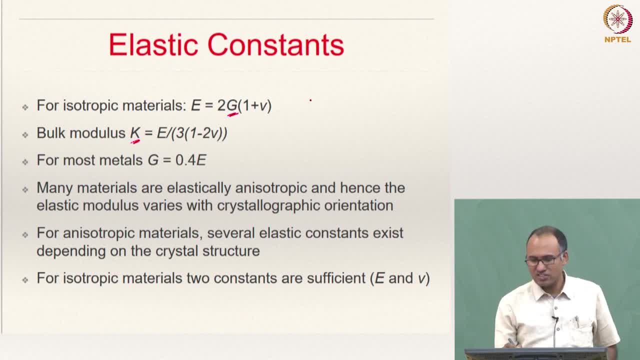 modulus K. So shear modulus relate shear strains with shear stress. tau is shear stress, gamma is shear strain and G is your shear strain. And bulk modulus connects what Pressure and volume, and all right, So you can always write a relation between these things and I am not going to derive. 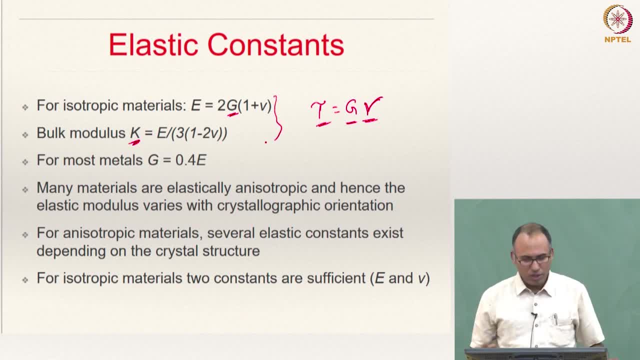 these relations, but I will leave it to your work so that you can derive them and then be happy about it. And for most materials, your Poisson's ratio is 0.25 or 0.3 and hence the relation between G and E is approximately 0.4..